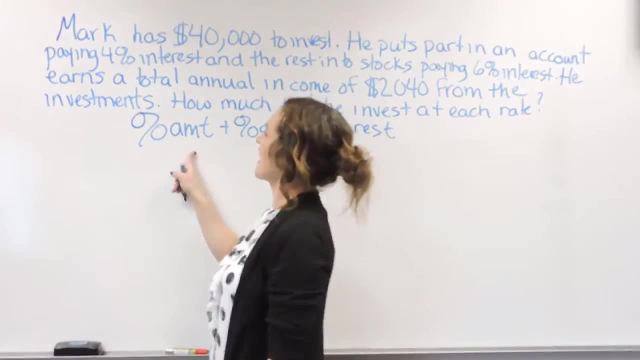 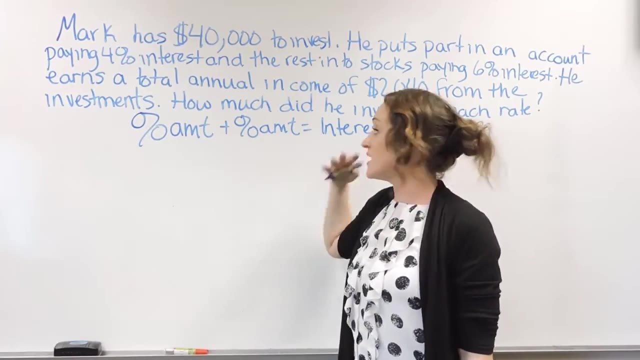 total here. So let's see He put some into this account at 4%. So do keep in mind, when we do plug in percent numbers into equations they do need to be converted to decimals. So 4% at a decimal here. 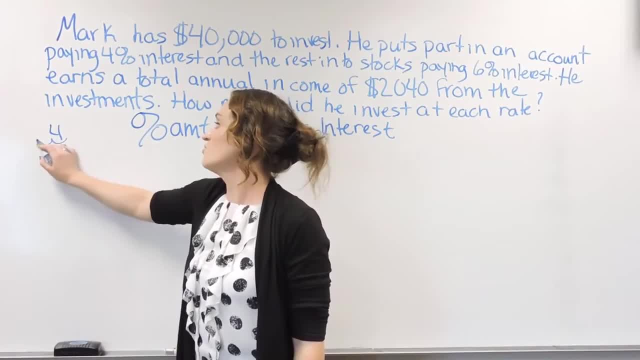 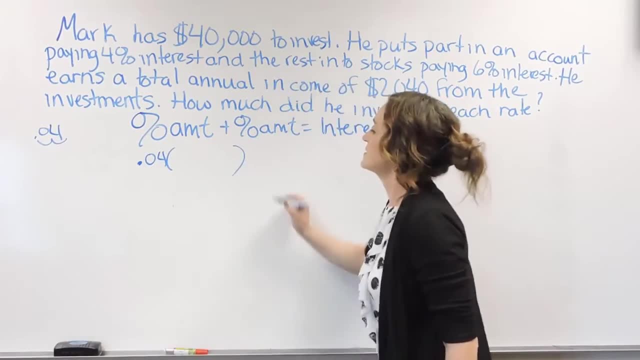 So remember to go from a percent to a decimal, You move that decimal two times to the left, So that would be 0.4 there times whatever the amount is. Then the other one is 6%, So that's going to be 0.6 times whatever that amount is, And it says that it's going to equal. 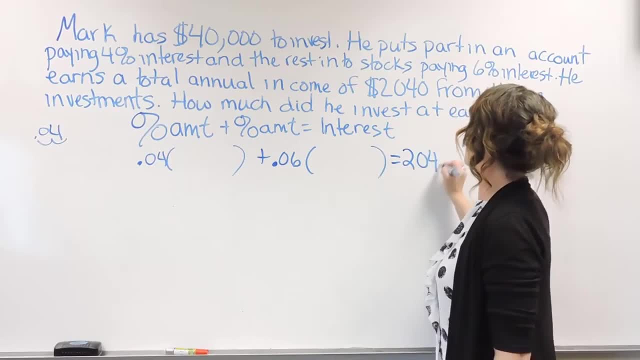 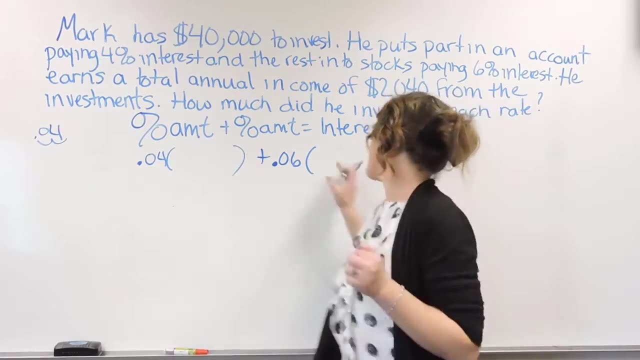 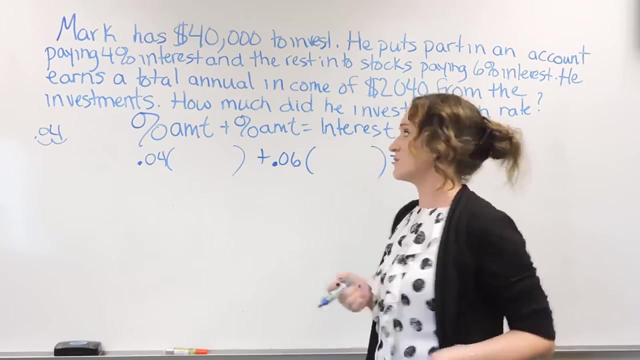 the total interest, And it said that he earned $2,040 in interest. So the only thing we really need to plug into this formula is we need to figure out the amounts here. Okay, so let's see Now one amount. Now we actually we don't know how much you put into the amounts. All we know is: 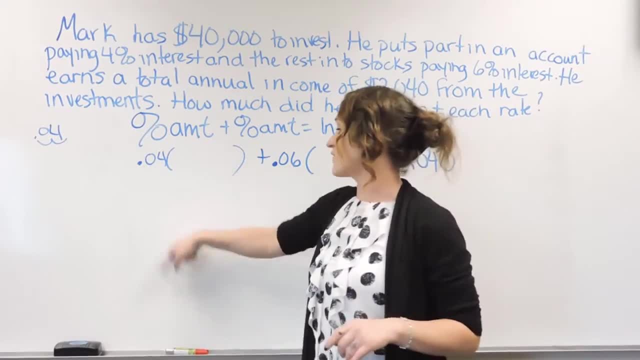 that together they add up to $40,000.. So we're going to plug in the amount here And we're going to put in $40,000.. So, whatever this first amount is here, let's just call it X, because we have no. 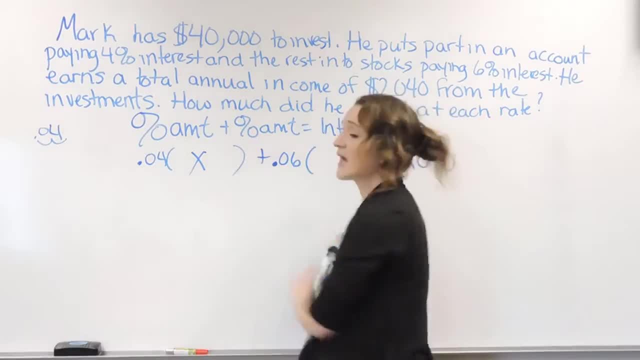 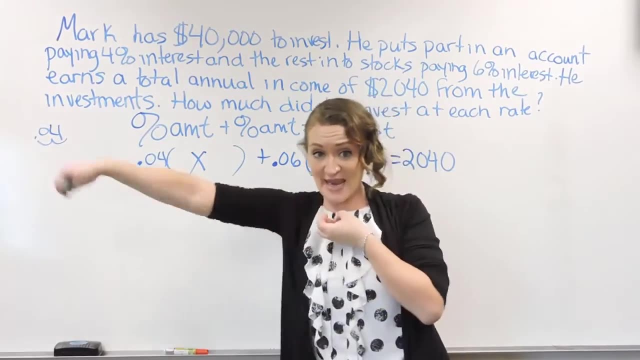 idea how much he put into one of them. All right, so he put X away into this one here. So if I had $40,000, but I put some away, so that means I'm taking out from that $40,000.. So, however much I 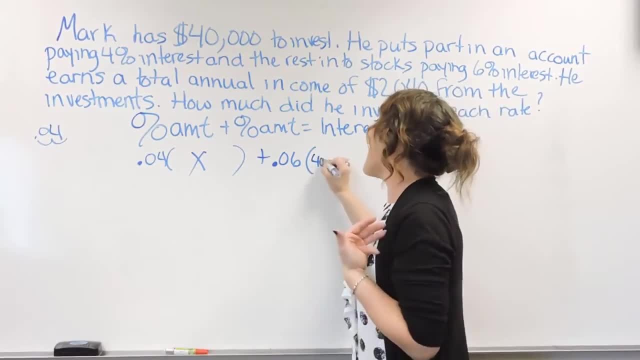 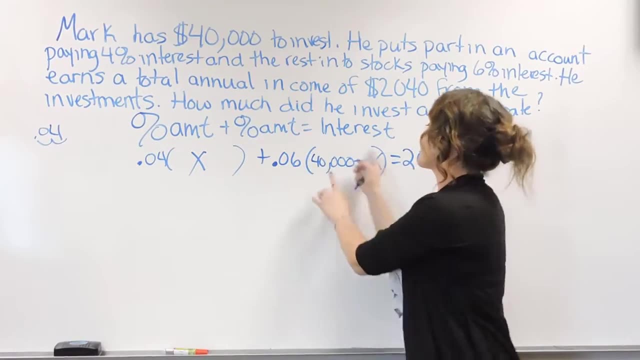 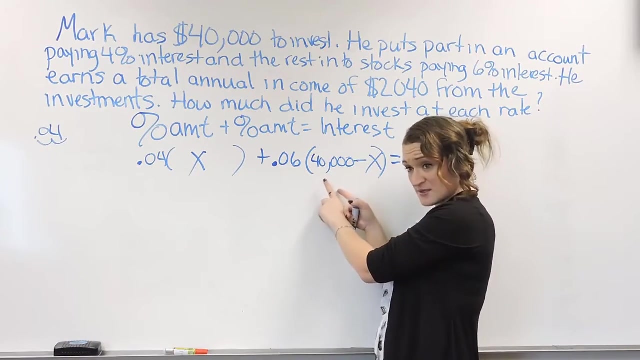 had left over and to go to this other account, I had $40,000, but I subtracted some X amount that over here. So this subtraction here what I had left over. after I took that out, that's how much I had for over here. right, I had $40,000 initially. I subtracted a bit to go over here, So this right. 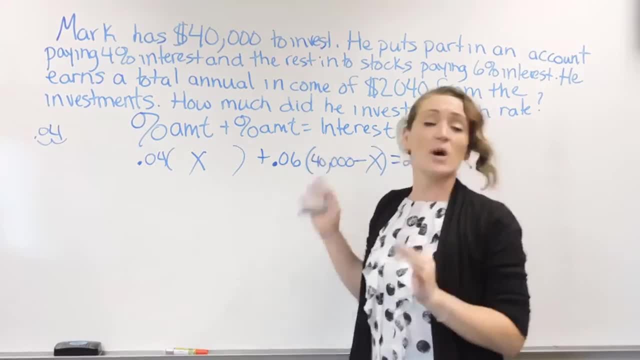 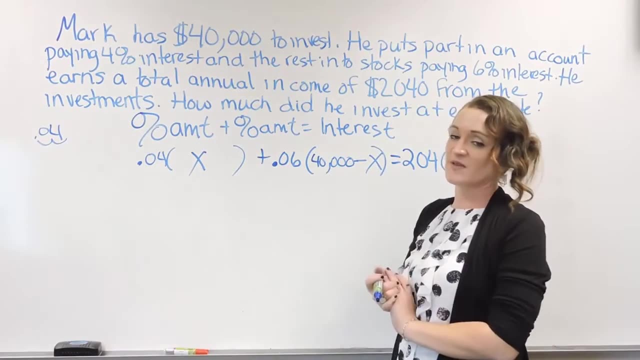 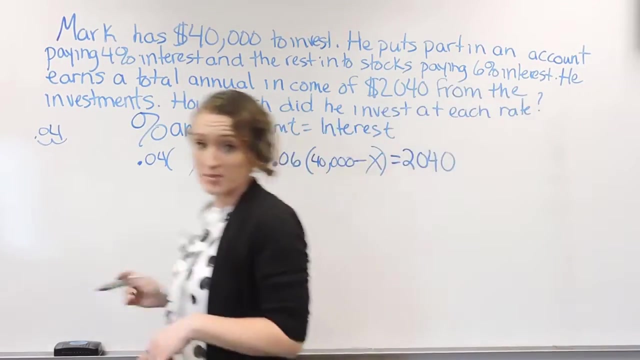 here represents how much I have left. So just pick one of them to be X, The other one will be your total minus X, And it'll work like this every time for these investment problems. So now that we have actually solved this problem, All right. so in order to solve this problem, let's see: 0.04X is. 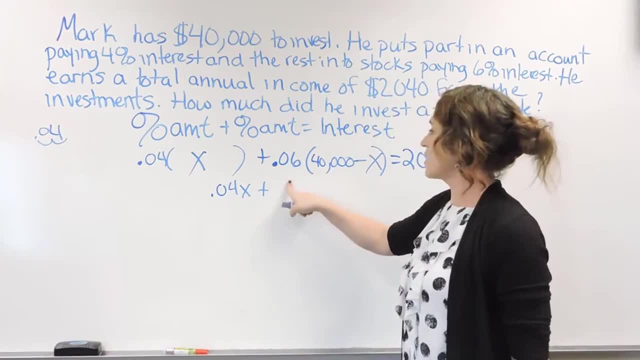 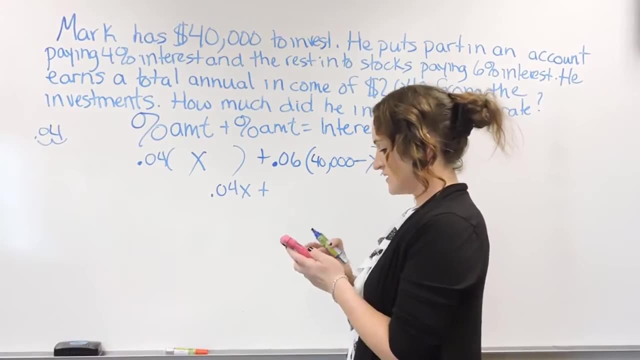 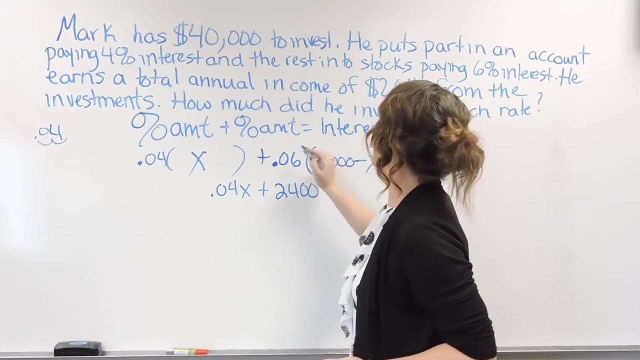 just 0.04X plus the 0.06 times $40,000.. Let me take out my handy dandy calculator here. So 0.06 times $40,000 is equal to $2,400 minus 0.06 times X. So we need to distribute that, It's just 0.06. 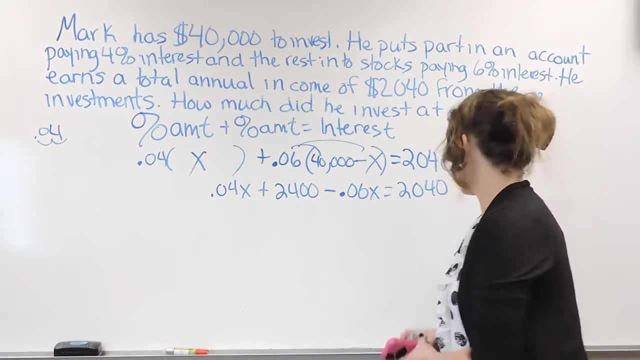 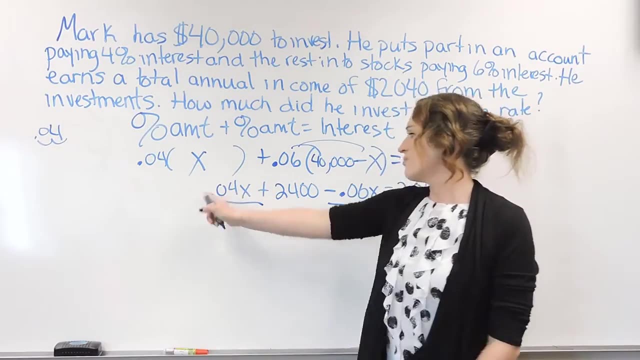 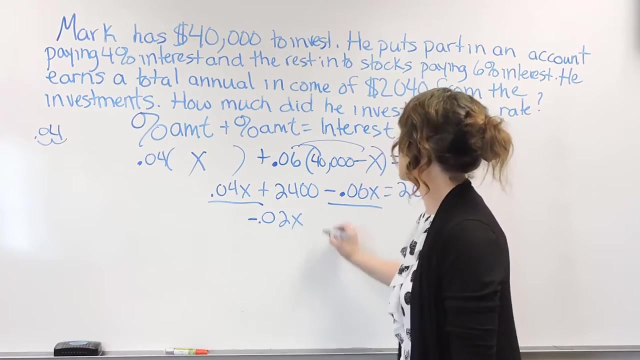 X, And this equals $2,040.. All right, so we need to continue simplifying here. Let's combine some like terms: 0.04X minus 0.06X. that's going to give us a negative 0.02X plus the $2,400. 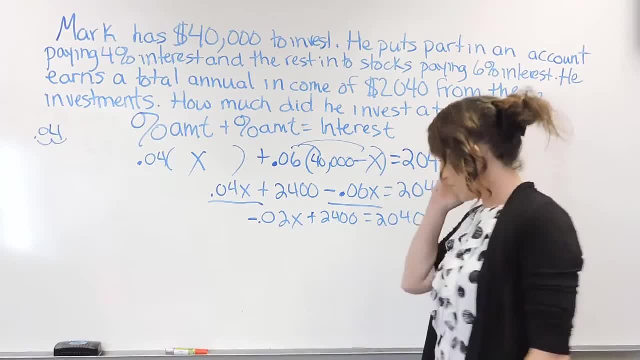 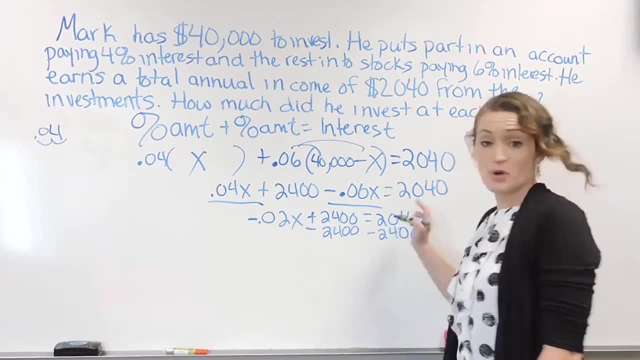 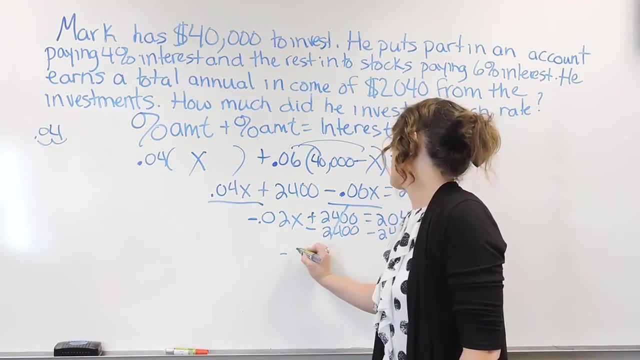 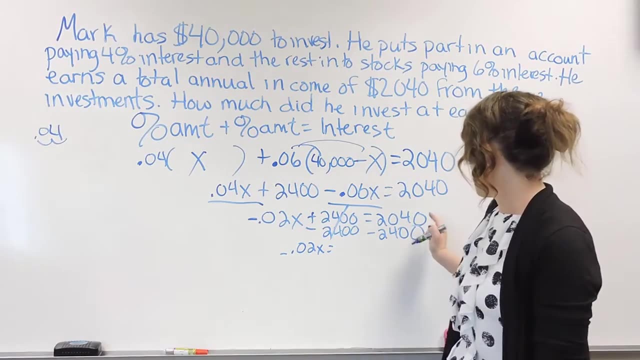 Both sides by $2,400.. That's going to cancel out over there on the left And we're left with 0.02X is equal to. so let's see here we're going to be left with $360.. All right, and divide both. 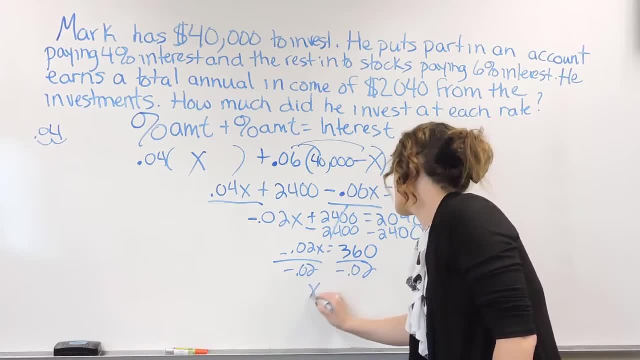 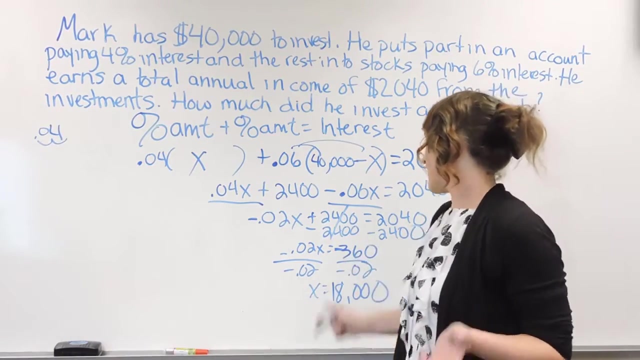 sides by 0.02.. And X is equal to. let's see handy dandy calculator here: 360 divided by 0.02 is $18,000.. All right, so that means that we put $18,000 in one account, the one that we labeled as X. 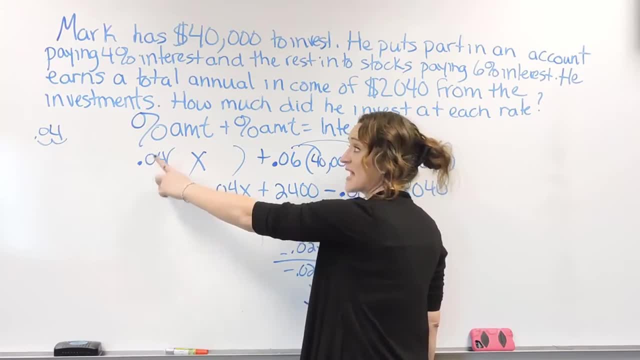 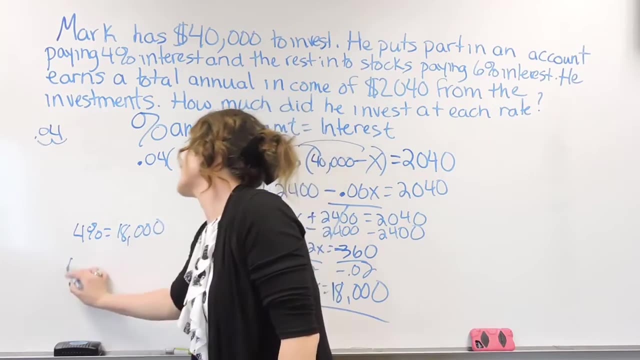 So X was the one over here at the 4%. All right, so at the account for 4% we put $18,000 there To figure out how much we put into the one at 6%. so this one right here represents our 6%. 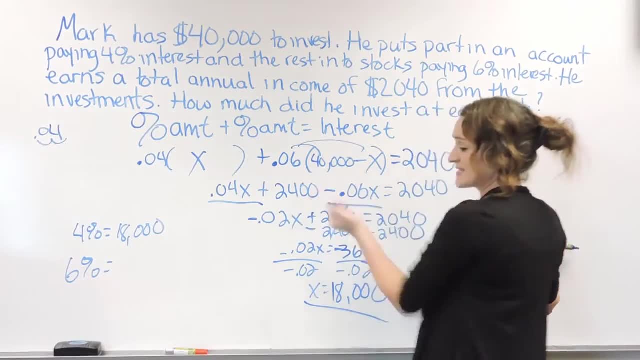 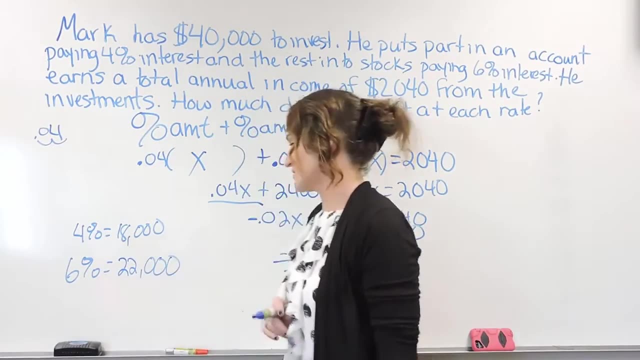 that was $40,000.. Minus that X, So if we take $40,000 minus 18, that's going to give us $22,000.. So $18,001, $22,000 in the other.